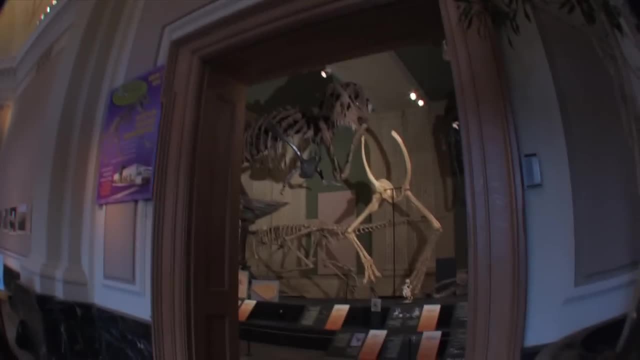 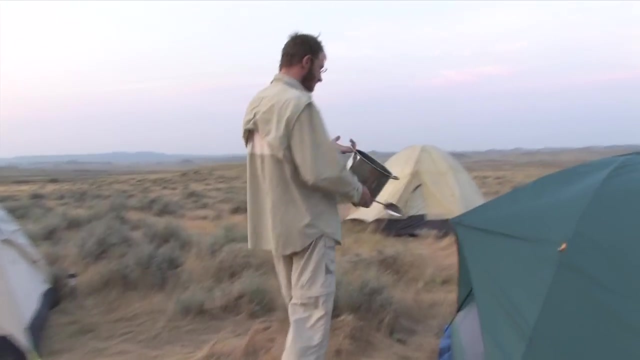 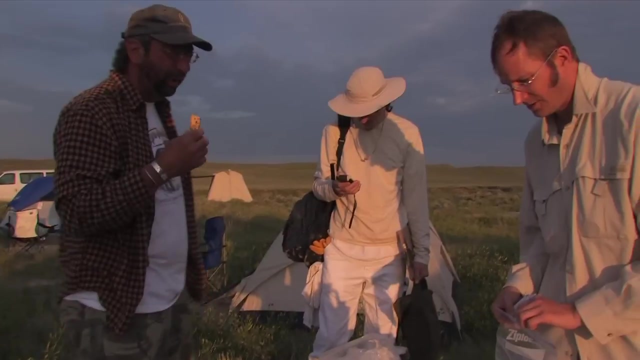 evolution. you'll see, those are the fossils we are after. I have learned a number of things from Dr Carr on these digs. One is that we have to start our day early, because it gets way too hot to work in the afternoon. Do you want coffee? 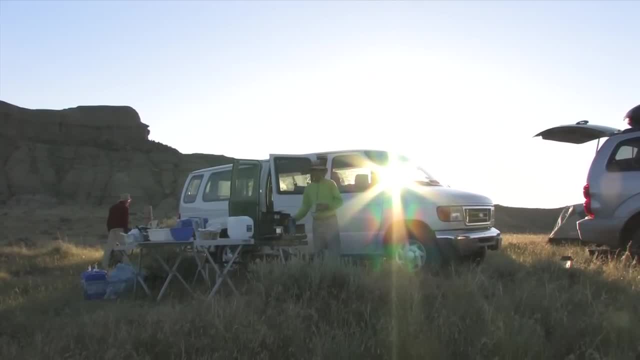 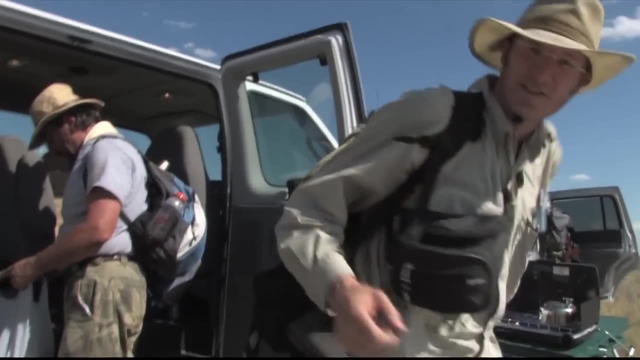 Please, Black. We also have to leave camp with everything we need, so there's a lot of prep work to be done. When we have all of our equipment, along with plenty of food and water, we are ready to head out for a busy and safe day. There are three major 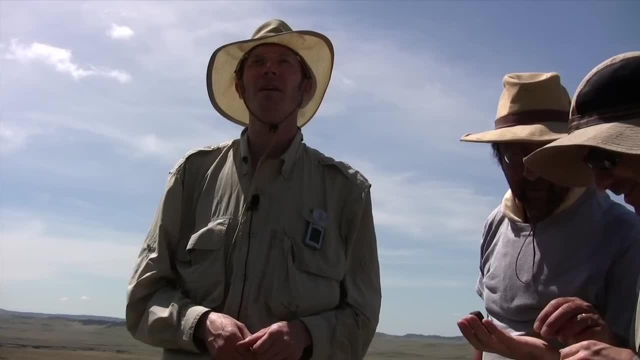 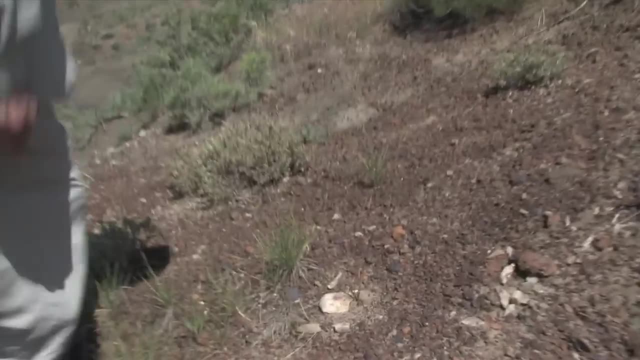 parts of a dig. The first is prospecting. Hey, look at that, I've gotten these up tangled. Prospecting is looking around or carefully observing your area for bone-like objects. Walking around the hillside, we look for scattered or possibly just a single bone or fragmentation. 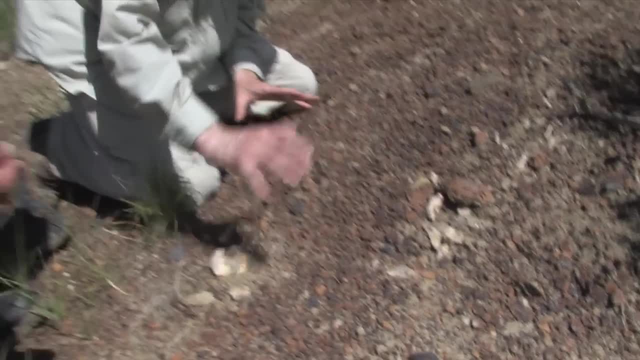 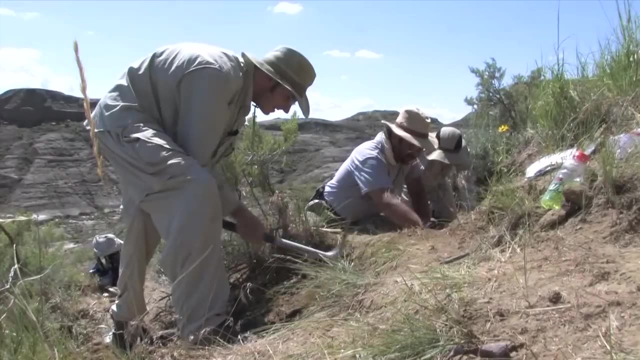 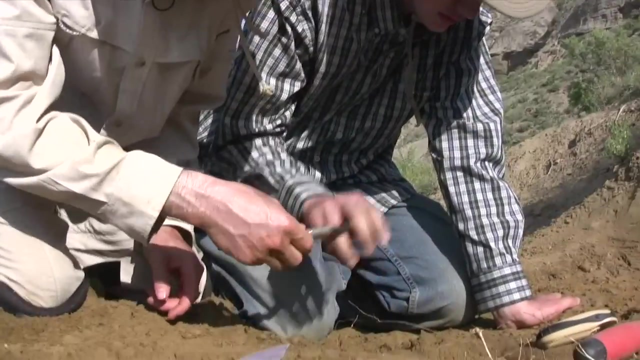 This is what I consider a scatter, and what we do is we follow it up, and there's more bone up there, so, who knows, it may continue further up. If we find something of interest, we look at it more closely. We carefully dig around the object, exposing it without harming or disturbing it. 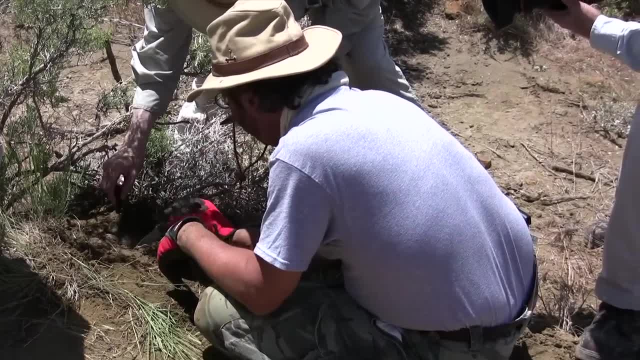 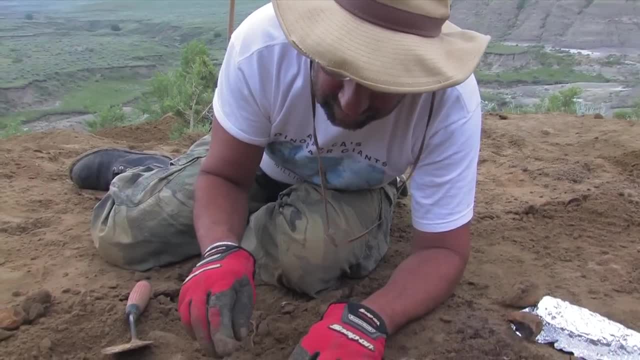 That's rock. Yeah, Sandstone, That's rock. Well, I might have found something else. It looks exactly the same. Obviously, this growth won't be hanging onto a rock, it'll be hanging onto a bone. so I'm 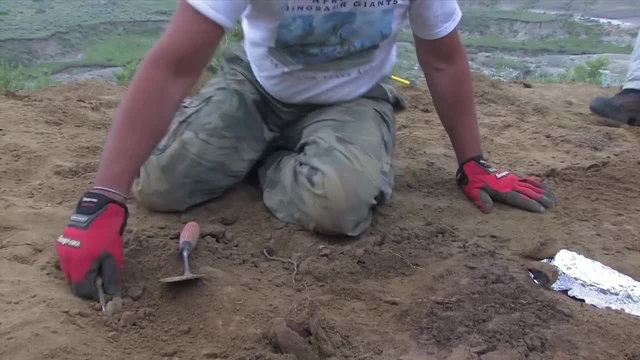 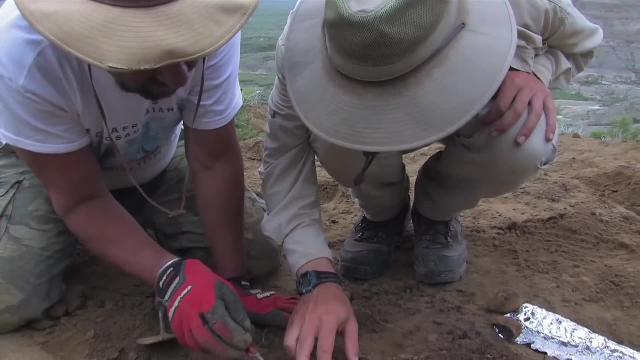 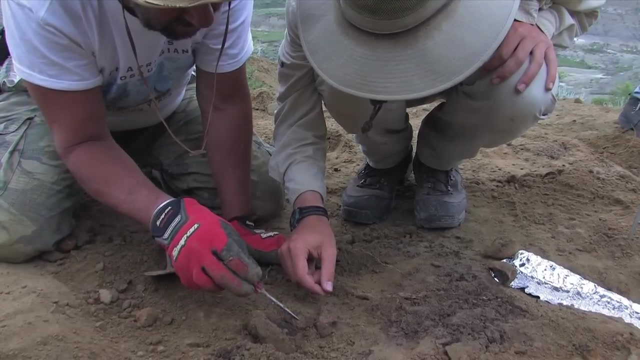 not sure. I think I should ask Eric to come over and take a look at this. Yes, Maybe. Yeah, I think so. Doesn't look like it. Yeah, This is usually the indication to me. is this growth on here? 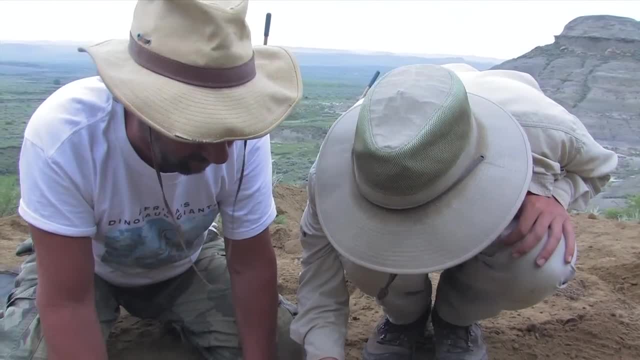 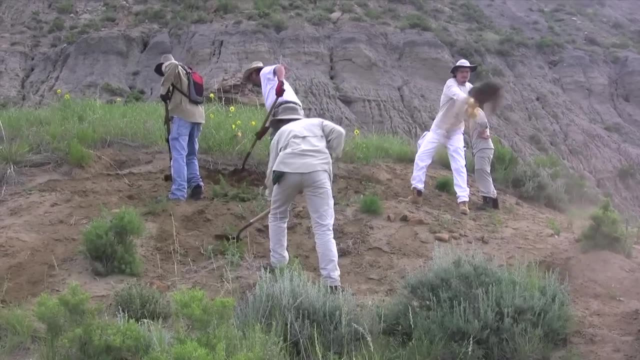 Yeah, That's a piece of bone. Yeah, It's definitely a piece of bone. Once something is identified as a bone, we start a process called quarrying. Quarrying is digging around the fossil to expose it and to see if there are other bones. 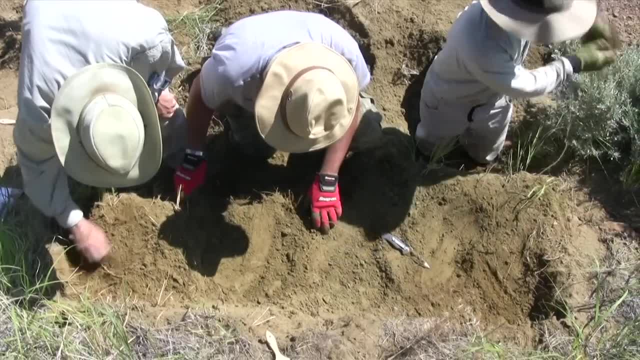 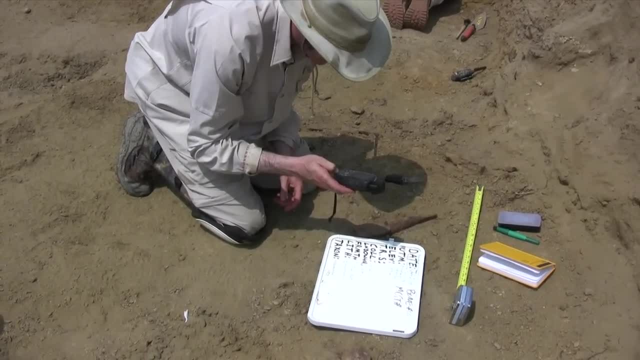 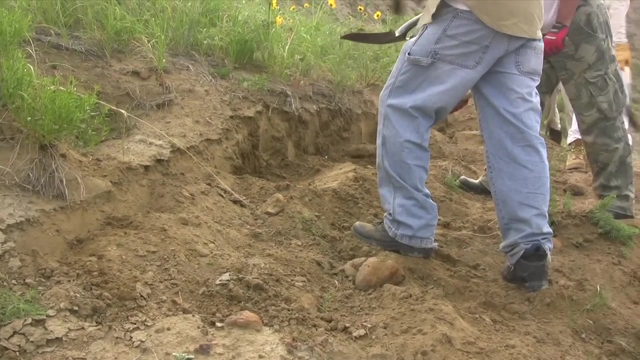 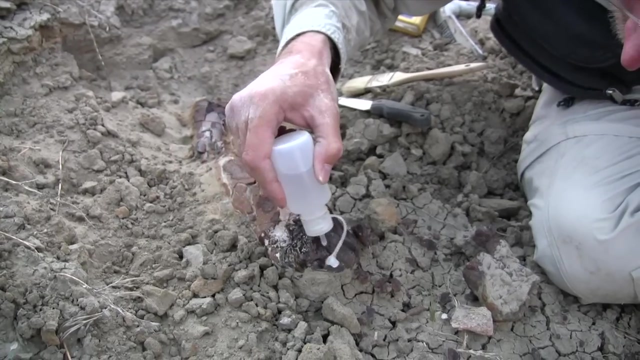 around. There are very important parts to this process, including first marking the object's exact location. We do this using GPS. This ensures that we always know precisely where the bone was found. then as much dirt as possible needs to be removed. We then apply coats of a liquid plastic called Vynac to stabilize the fossil. 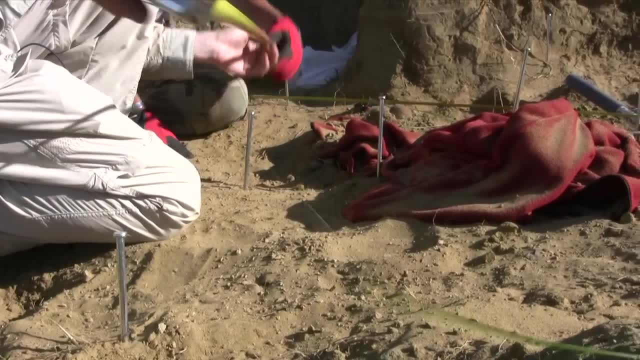 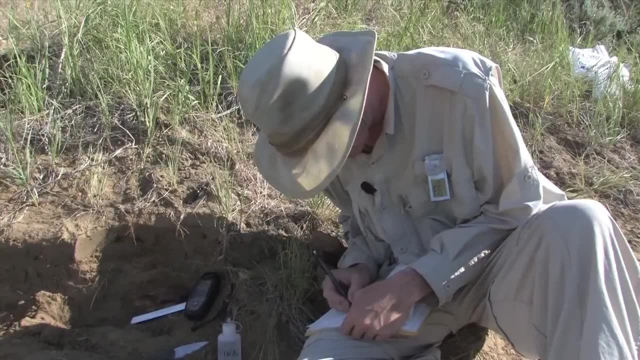 The site is also mapped before removing any bones, which helps pinpoint their relationship to one another, And this brings up a good point. During a dig, we log or take notes on everything. It is important to have documentation on all aspects of fossil digs. 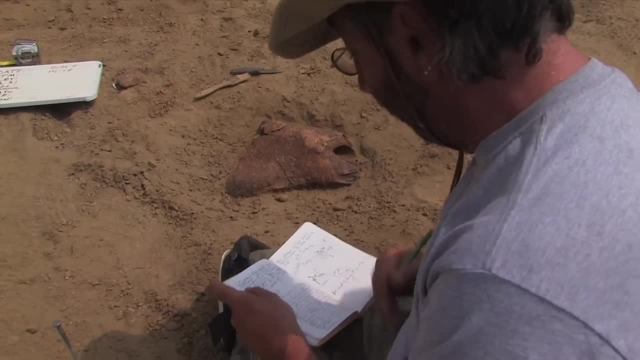 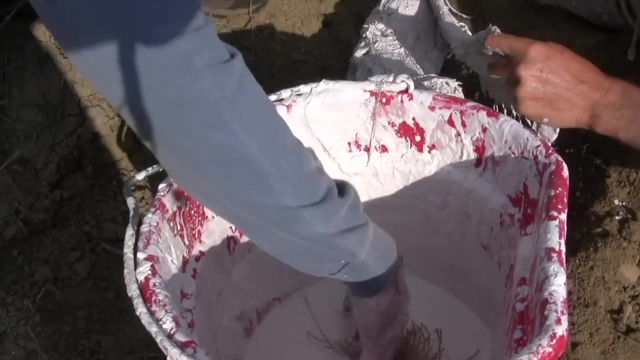 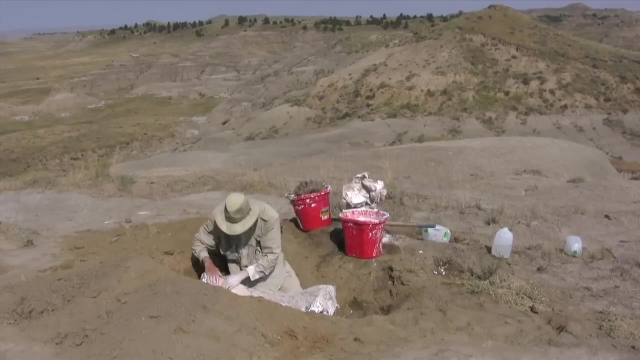 I'm just kind of taking some notes on what we did yesterday. After the fossils are stabilized, GPSed and mapped, they are wrapped in a messy but sort of fun process called jacketing. Jacketing ensures that each specimen is protected as much as possible. 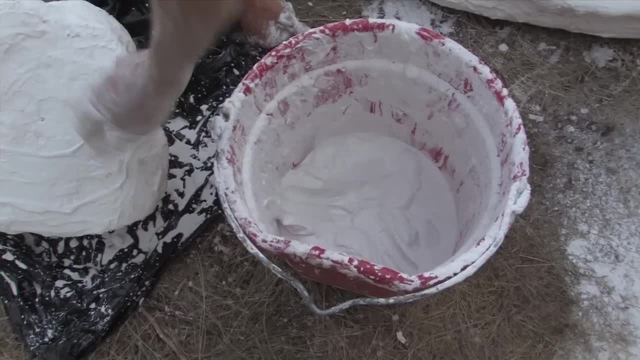 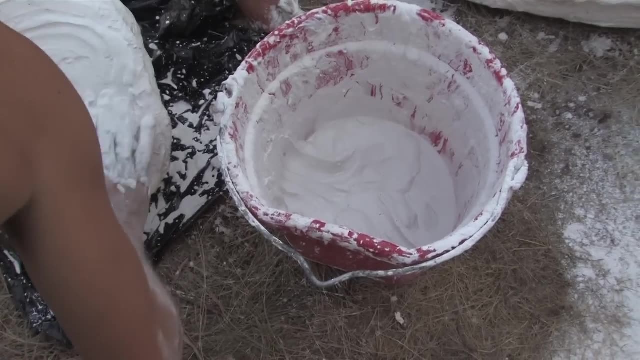 We encase the bone inside a plaster jacket. When the top half is dry, the fossil is rolled over and the jacket is completed. The jacketed fossil bakes for about a day in the sun And is then ready for transport. Some jackets get very heavy. 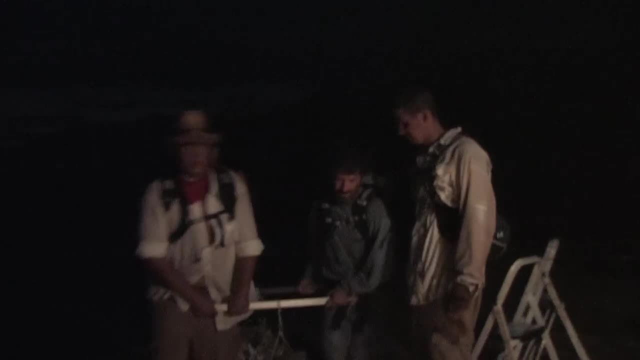 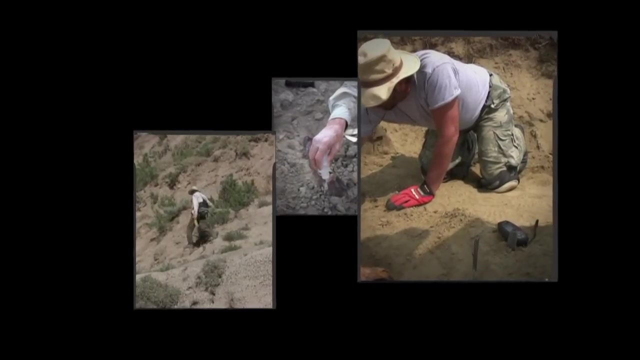 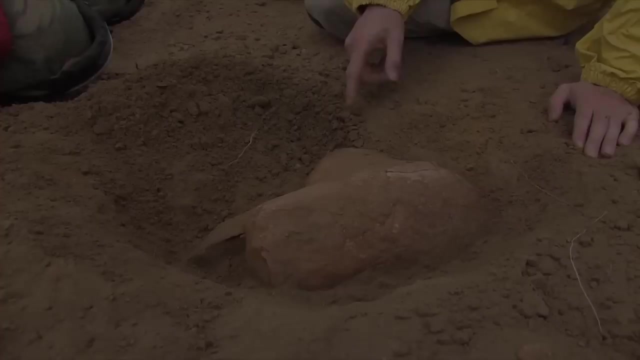 We had to carry this one back in the evening to avoid the heat of the day. The step-by-step procedure of a typical find- prospecting, quarrying, Vynac-ing, mapping, jacketing and finally extraction- aids in not only preserving the bones but preserving 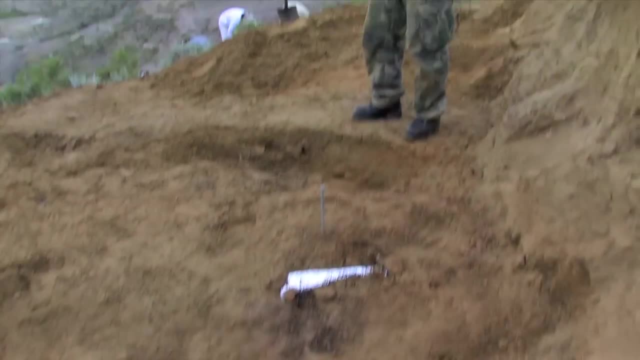 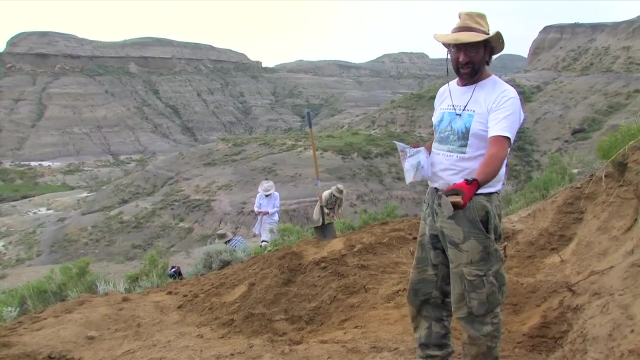 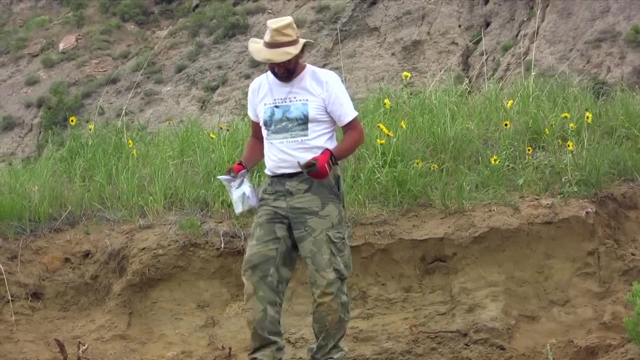 and understanding what the bones and their location can mean. So I'm definitely ending on a good note. It's pretty exciting. I mean any time you find any little thing it's exciting. but being in the same grid with the, with the portion of the female we found last year, that's pretty exciting, pretty. 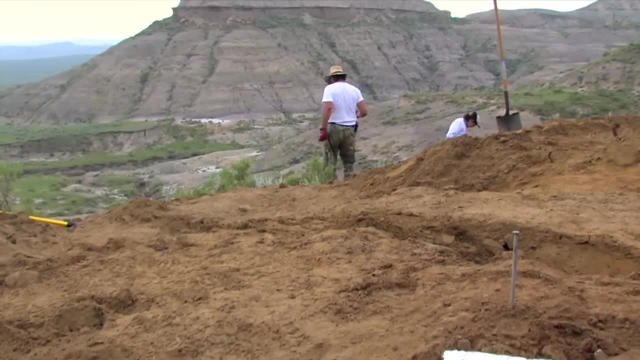 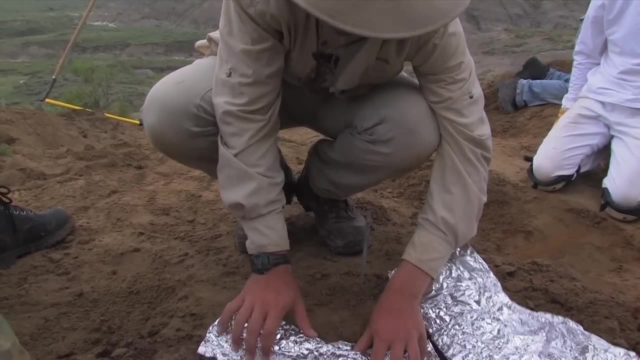 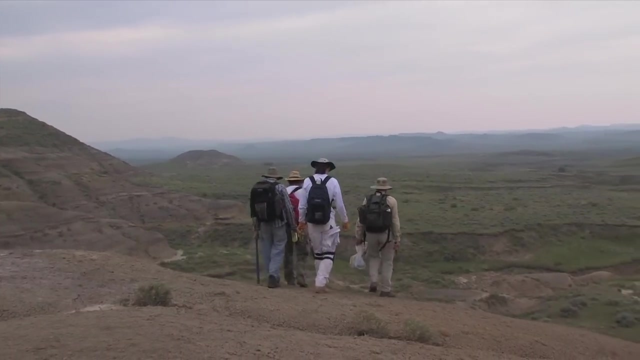 exciting. After long hours of digging, it's time to call it a day. We make sure our fossils are covered to protect them from the weather, so we can pick up where we left off. We grab our personal items and head back to camp.